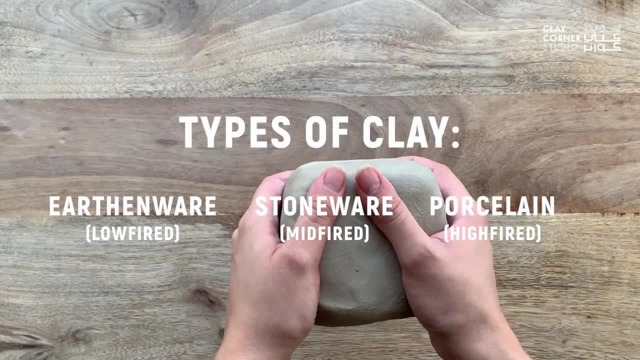 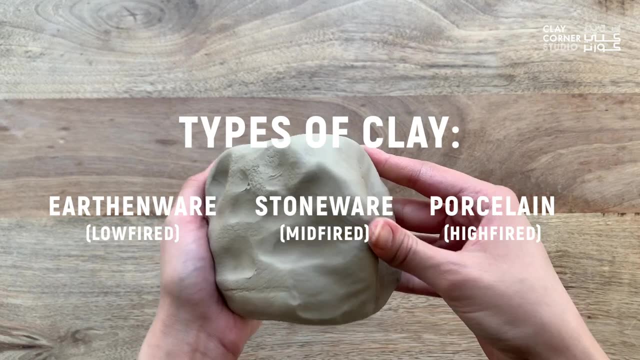 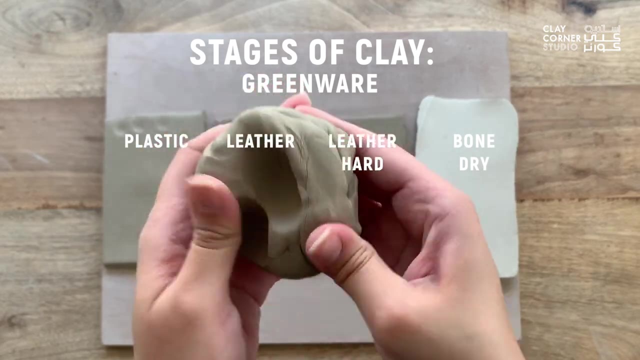 Natural clay comes in three main ranges: earthenware, which is low fired, stoneware, which is mid-fired, and porcelain, which is high fired. Each of these types of clays go through different stages as they dry. When the clay is soft and malleable, it is called plastic clay. 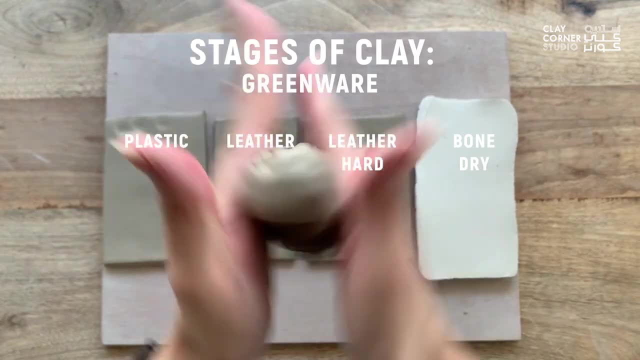 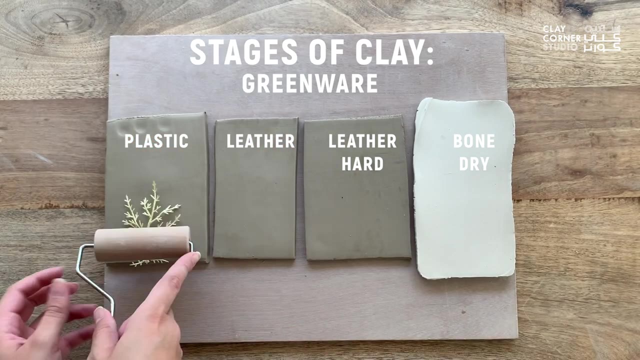 because you can easily bend it and work with it without breaking and cracking. Plastic clay is ideal for coiling, pinching and wedging and can take on texture very well. Keep in mind that soft clay is not wet clay, As it dries a little. 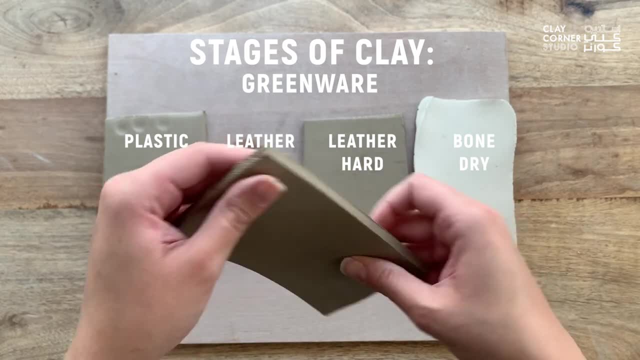 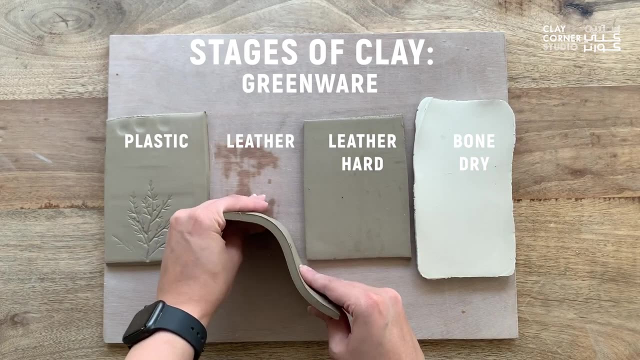 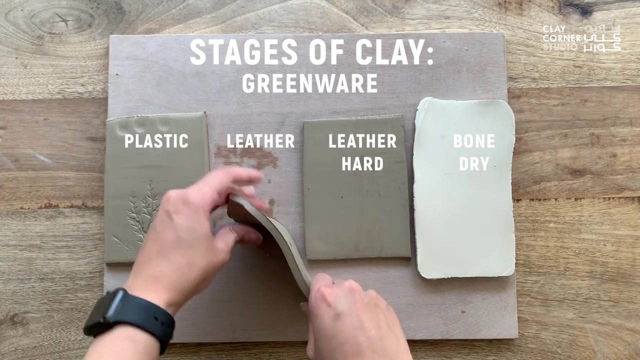 the clay enters the leather stage when it is no longer sticky to the touch and can hold its shape when standing upright. At this stage, you can still get away with shaping it and bending it a little without cracking. Leather clay is ideal for slab building and for scoring and slipping. 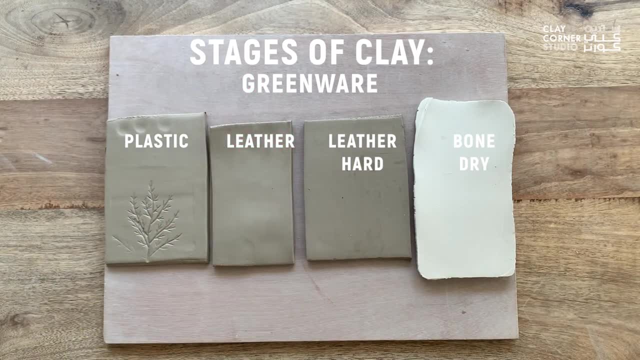 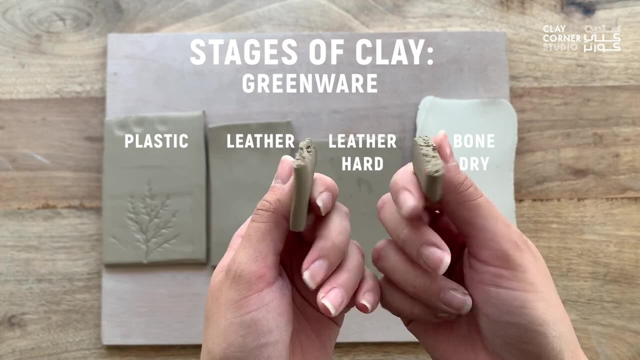 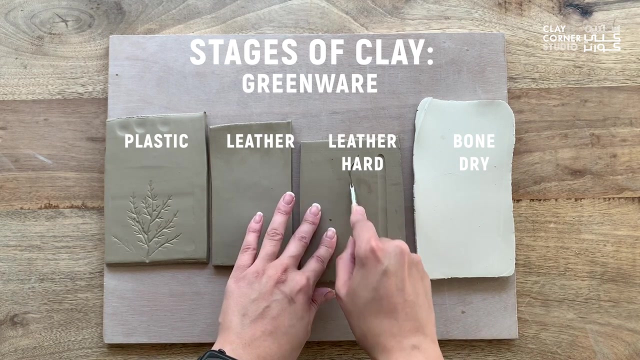 or in other words, attaching two pieces together. The next stage is leather hard, and it is when the clay can no longer be bent, but it is not yet completely dry. This stage is great for cleaning up and polishing the piece, such as smoothing it down with a wet sponge or trimming and carving. 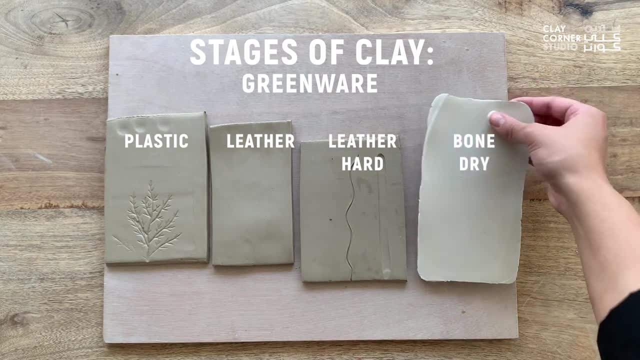 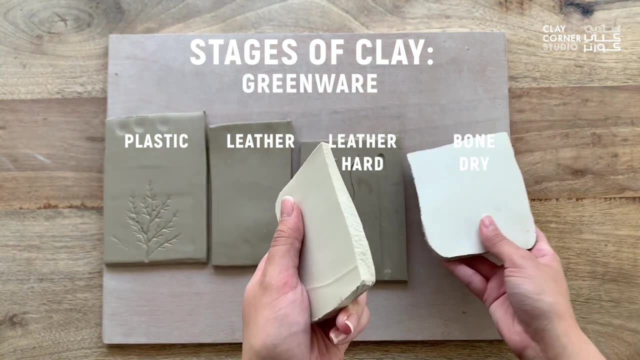 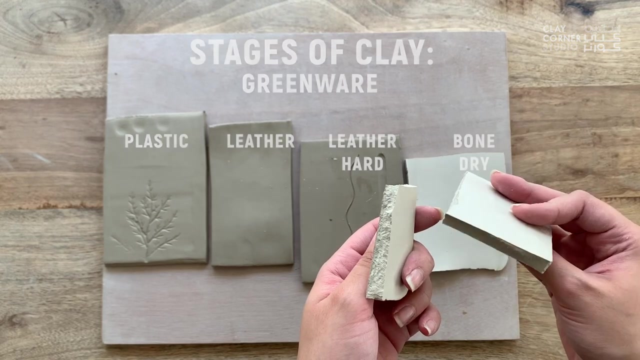 When the clay is completely dry, it is called bone dry. At this stage, you can no longer bend, attach or shape it. However, you can still buff and sand it. The piece is quite fragile at this stage and not functional until fired. One use for bone dry clay is making slip. 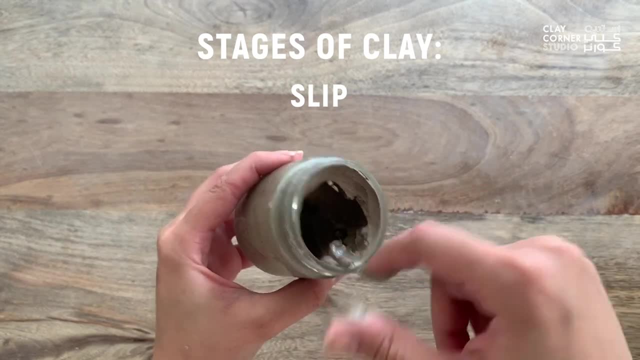 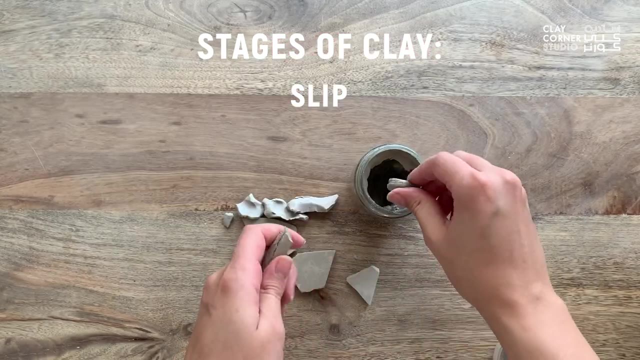 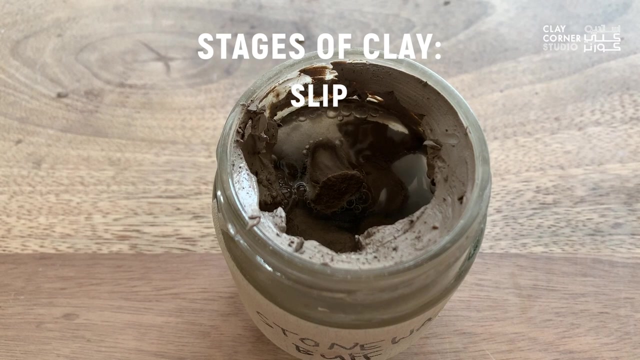 Slip can be used to form the clay which is made using bone dry clay and water, since bone dry clay absorbs water much faster than any other stage of clay. Slip can be used like glue to attach pieces of clay together, or sometimes be used to slip cast into plaster moulds. 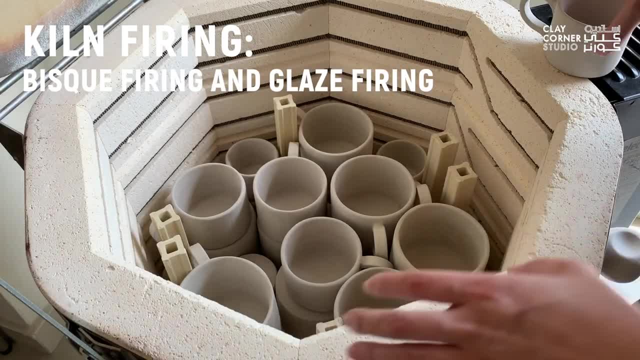 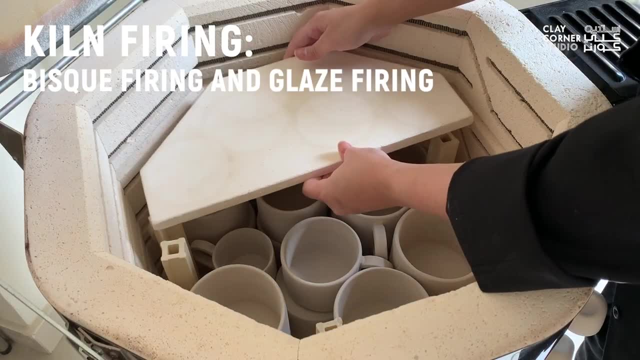 Pieces made with clay in all its stages before firing are called greenware and are not yet ceramic pieces. The first firing that clay goes through to become ceramic is called a bisque firing. Ceramics are fired in a kiln, which is an oven made for ceramics. 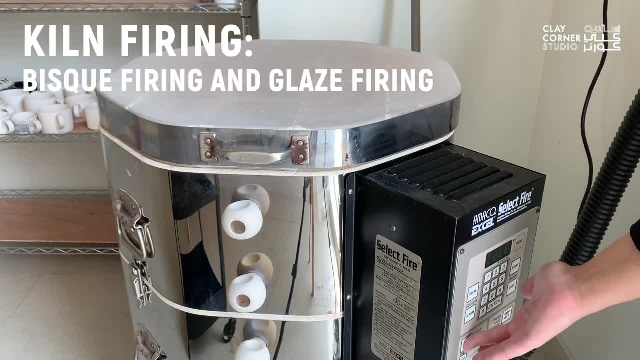 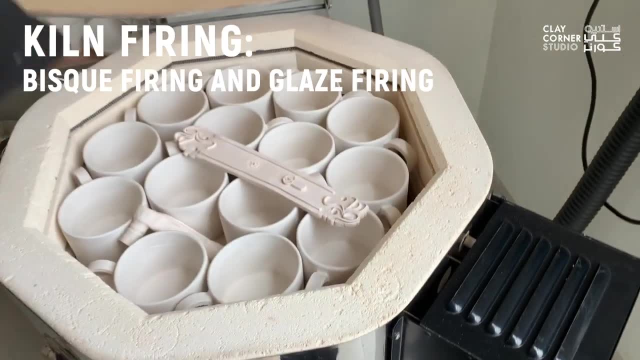 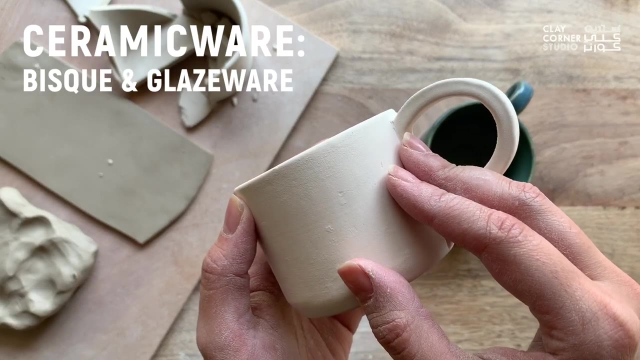 that fires to very high temperatures of over 1000 degrees Celsius. Firing can happen at different ranges for different types of clays and glazes. Once bisque fired, the unglazed ceramic piece is called a bisque and it is not yet functional or food safe until it is fired. 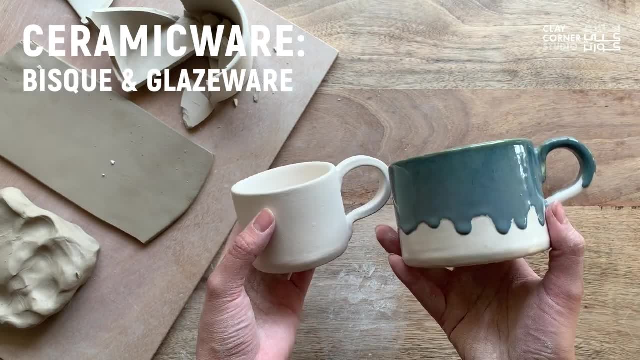 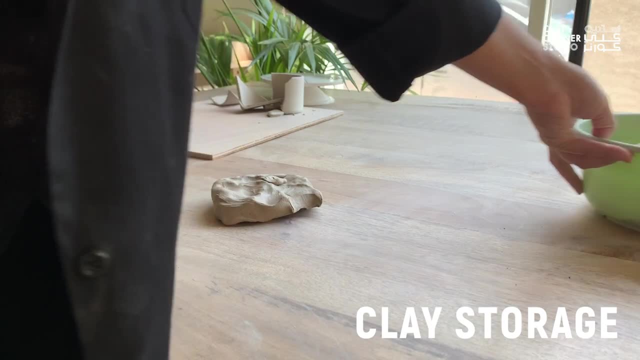 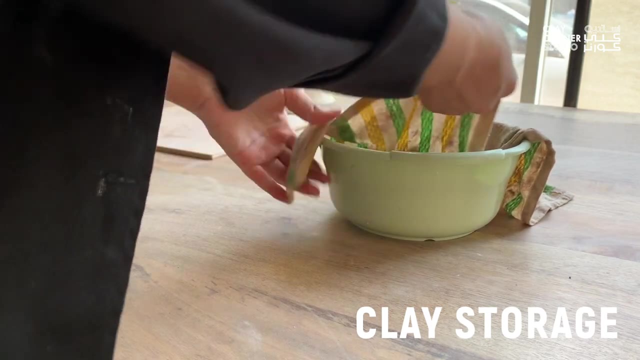 It is glazed and fired again After glaze firing. you now have a completed ceramic ware. When clay is left exposed to air, it will naturally dry out. So to keep your clay moist and soft, it must be stored in a damp and airtight container. 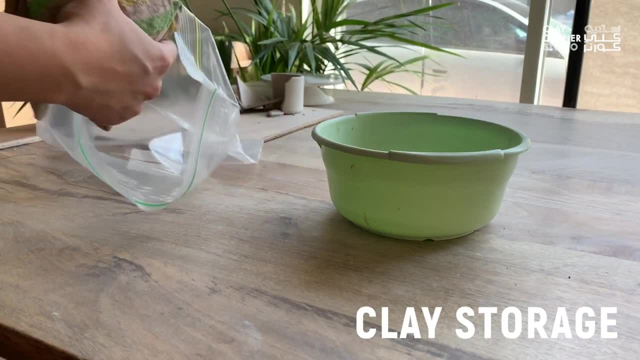 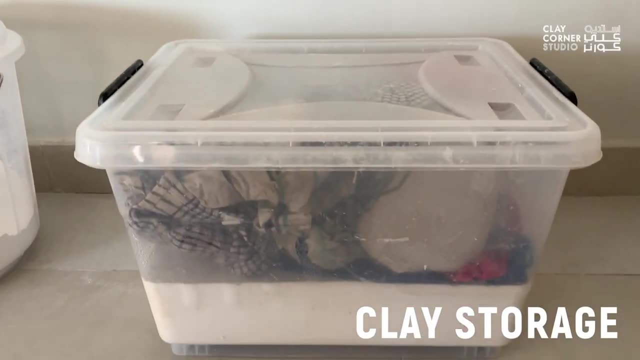 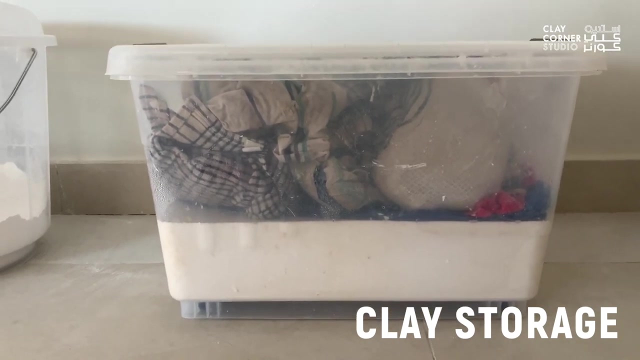 such as a ziplock bag. If your clay has hardened a little, you can also wrap a damp cloth around it to rehydrate it before sealing it in the bag. Another option is to store your clay in a damp box which has been filled a quarter of the way with plaster that has been saturated with water. 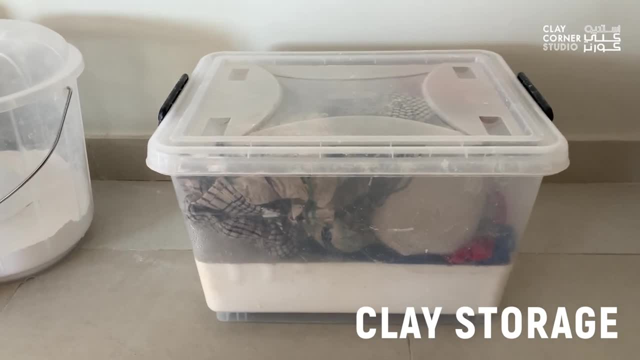 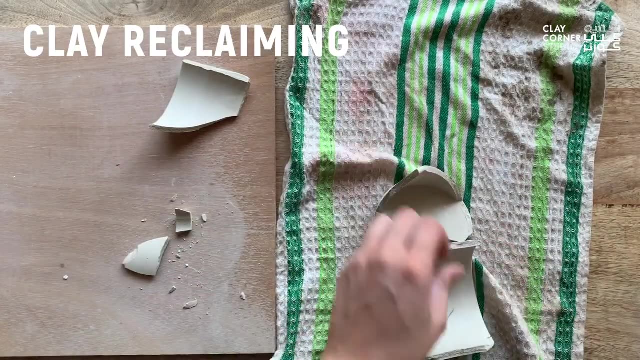 which creates a humid environment that is ideal for keeping the clay soft for weeks or even months. To rehydrate bone dry clay, you can either place it in a wet kitchen towel and in a ziplock bag and allow it to slowly soak in the moisture over the next several days. 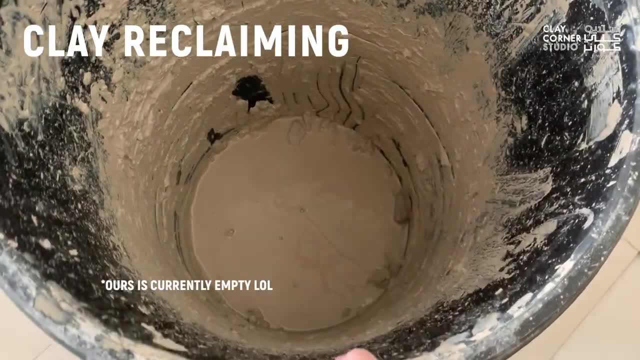 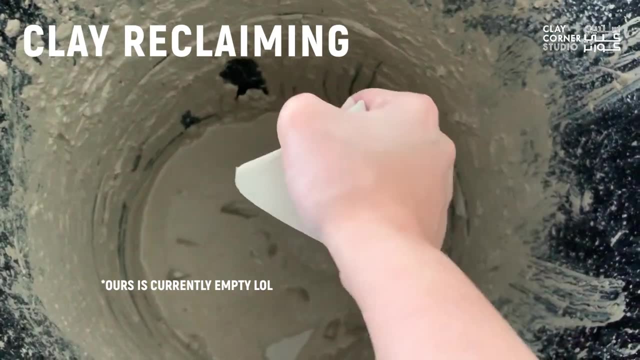 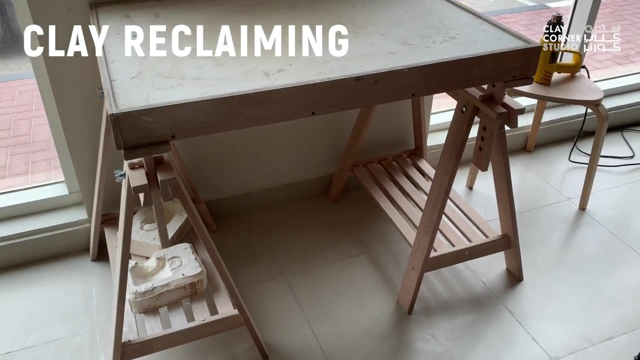 or you can reclaim it by turning it into slip. first, You'll often see a clay reclaiming bin in ceramic studios where you can throw in your bone dry clay to recycle. When the clay has turned to slip, it is then spread on a plaster surface to dry out until it reaches the plastic stage. 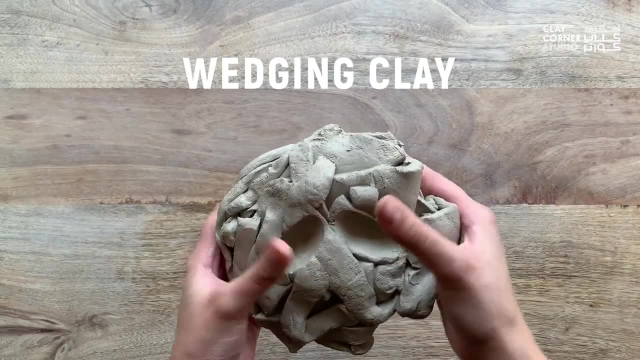 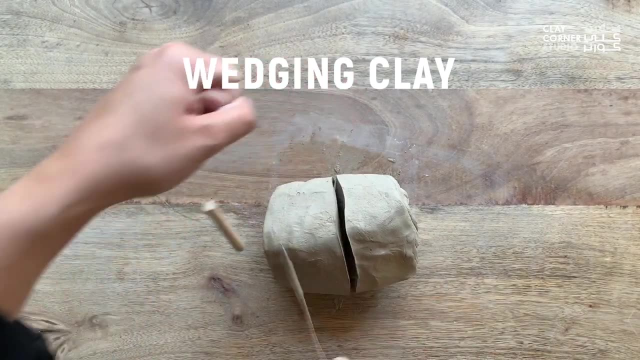 Before using any clay to create your masterpieces, you must wedge the clay first to release any air pockets that might be trapped inside it. This is very important because trapped air can shatter the piece in the cone or create stresses or weak points in your ceramic pieces. 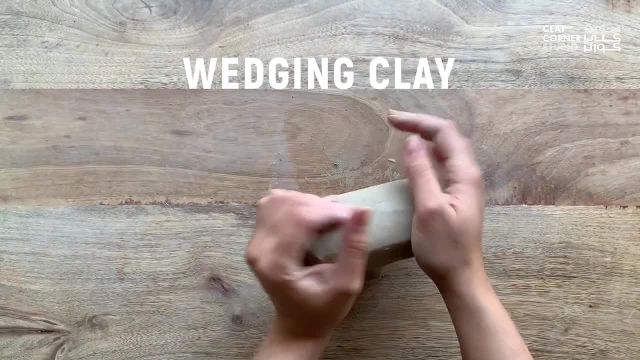 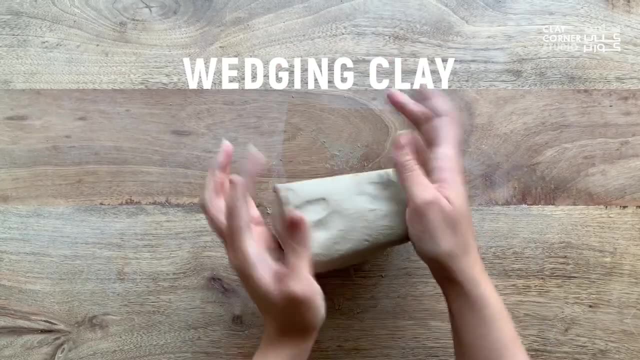 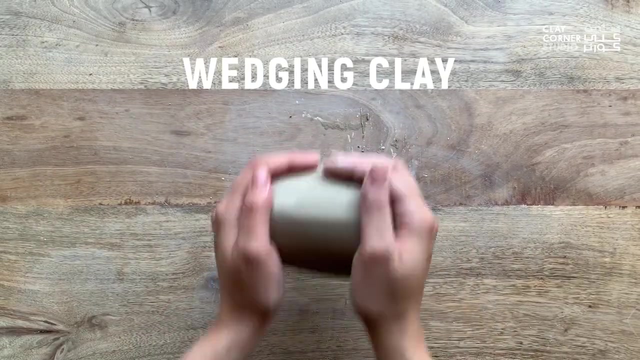 There are different ways to wedge your clay, and the method shown here is called a ram skull. You need to make sure that you do not fold in your clay, because that can create new air pockets. The goal here is to knead the clay very gradually, to turn it inside out until all the air inside it. 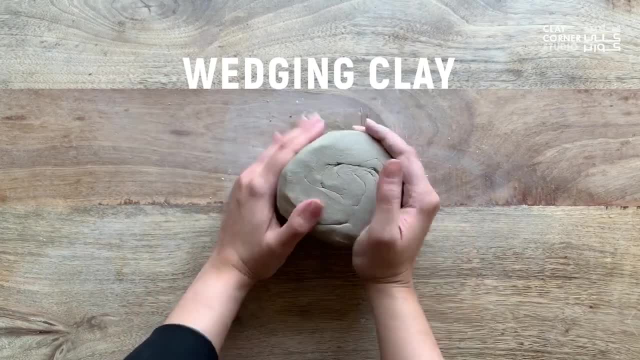 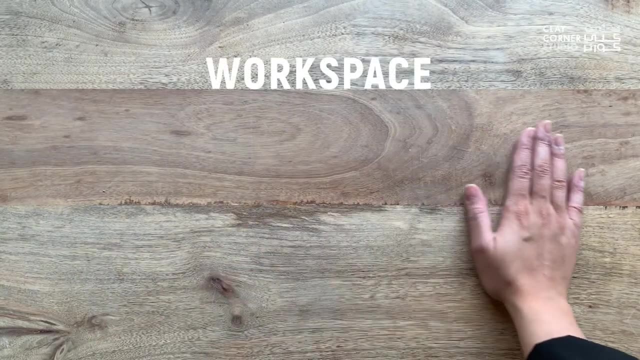 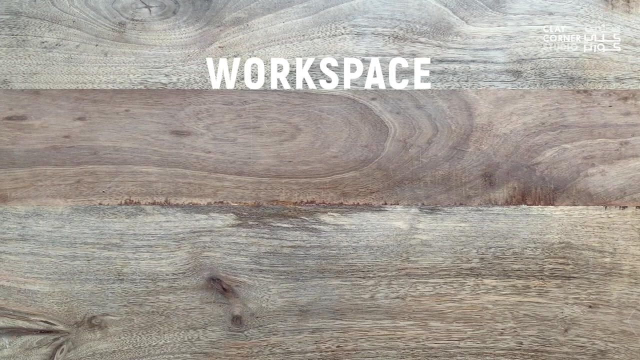 is released, And you must be careful not to strain your wrists while wedging. When working with clay, it's important to use a non-stick surface. Clay will stick to non-porous or polished surfaces like plastic, glass or metal, so instead you can work on an unpolished wooden table. 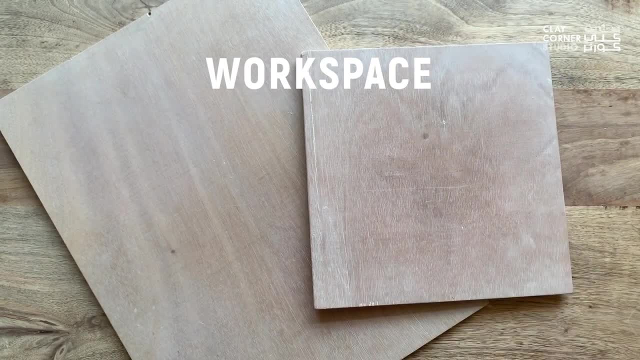 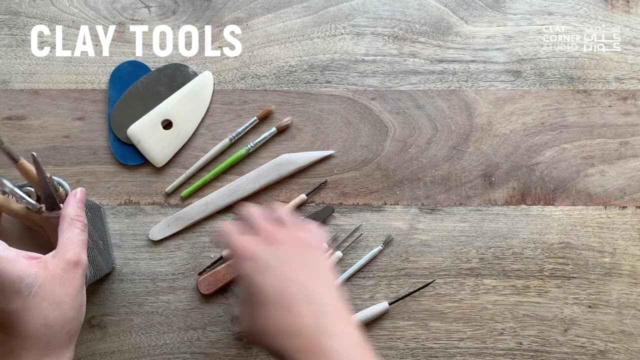 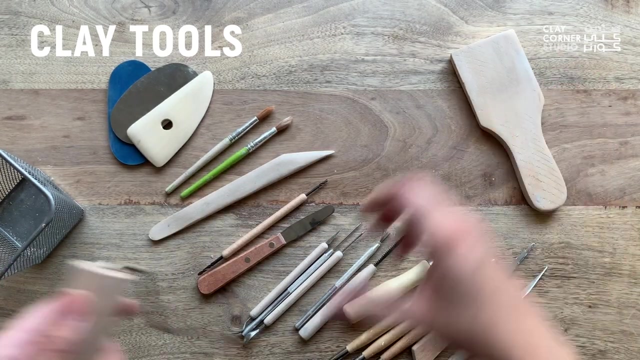 If you don't own one, then you can cover your table with unprimed canvas or use pieces of plywood to work on. When it comes to using clay tools, there is always more than one function that you can use each for. Just go with your instincts and see what fits the purpose you need. 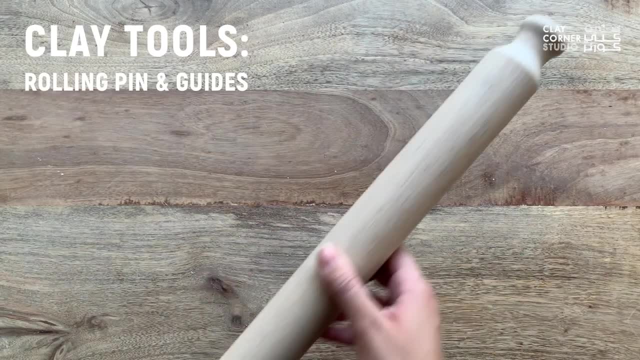 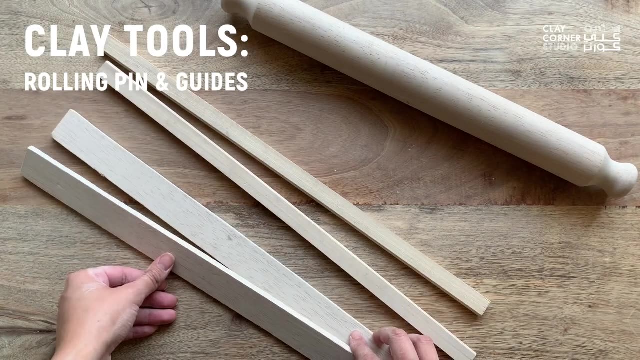 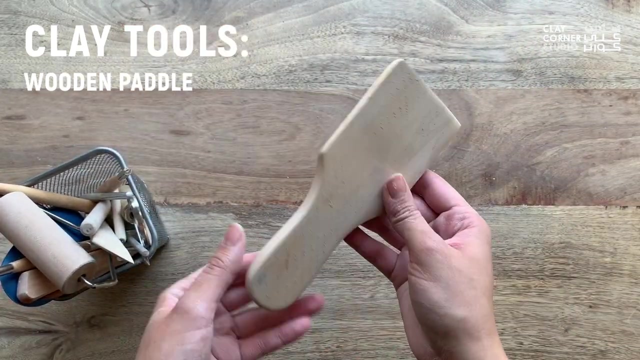 Here are some examples of basic tools that you can have: A rolling pin and rolling guides to create slabs. Rolling guides can come in different thicknesses and help you maintain an even thickness throughout your piece. A wooden paddle is handy in manipulating the shape of a clay object by using it. 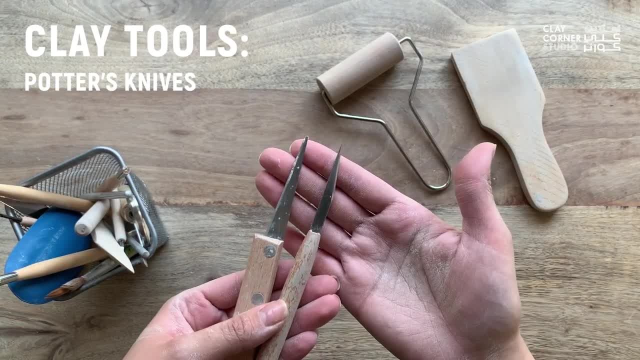 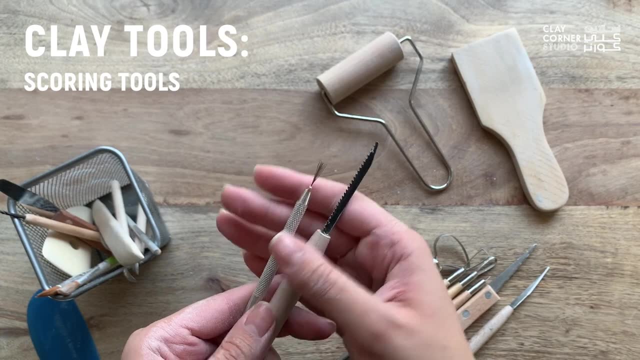 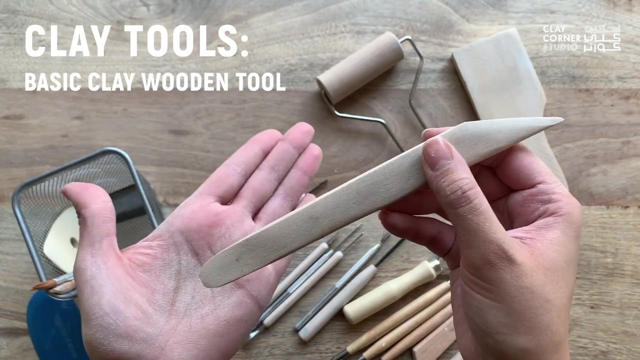 Patting it down. Putter's knives to cut the clay. Different ribbon tools to carve your piece. Scoring tools to score your clay before applying slip and attaching pieces together. Pin tools and shaping tools for details. Your basic wooden clay tool, which is very versatile and can be used to smoothen edges. 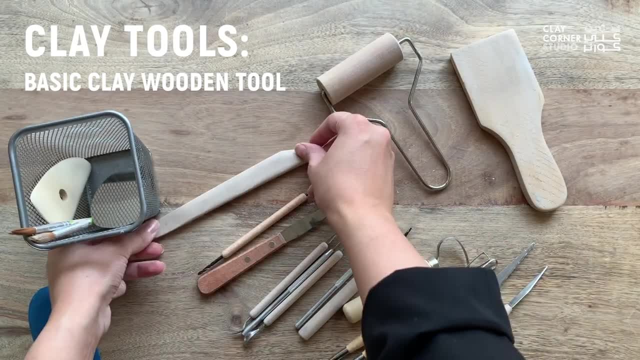 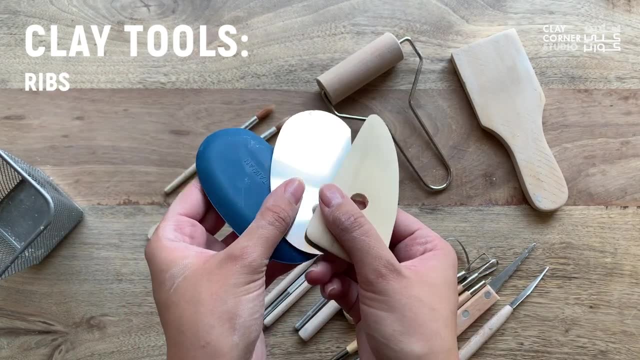 reach into hard-to-reach spots, shape or engrave into your clay Brushes to apply slip or water or smoothen Any joints. Ribs are used to smooth the texture and compress clay slabs and can come in wood, steel or rubber. 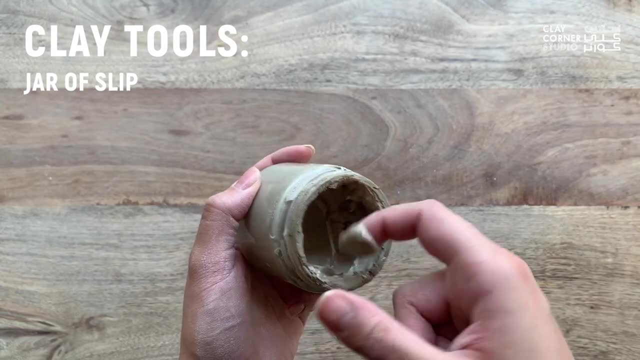 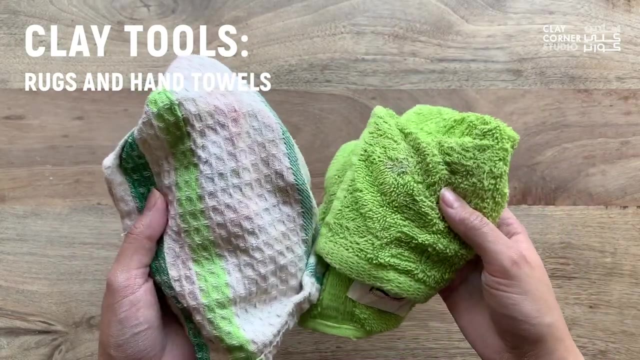 Having a slip jar made from the same clay body that you use in your studio is a must if you're joining pieces of clay together. It's a good idea to have rugs and hand towels about in your studio for cleanup and other purposes. A wet sponge helps you smooth your clay. 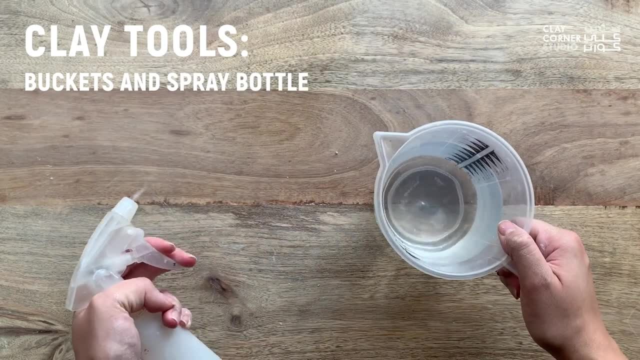 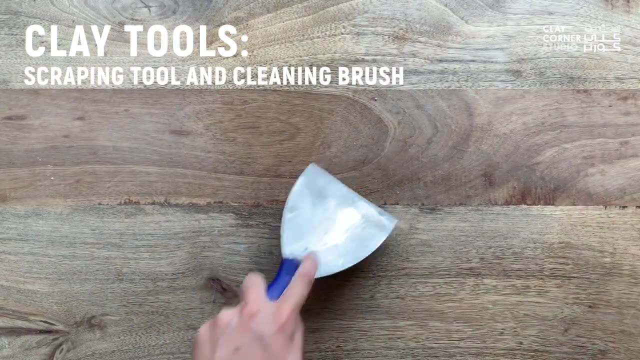 You'll often need a small bucket of water and a water spray bottle. You'll also need a hand towel to clean up and rehydrate your clay. To clean up your surface. a scraping tool and a hand brush are good to have in your studio.